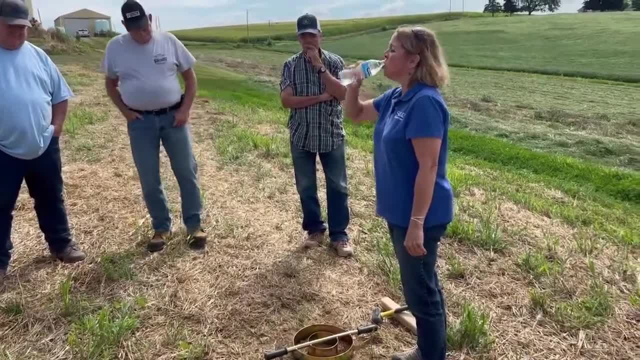 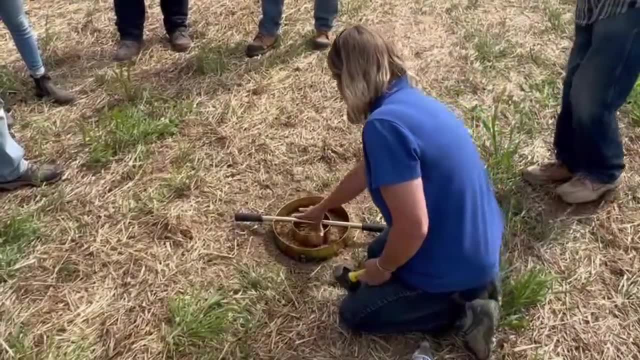 But what you do? a big swig of water that gets you about the right amount of rainfall to simulate an inch. So you're going to set your ring down. You don't want to hammer directly on the ring, if you can help it. 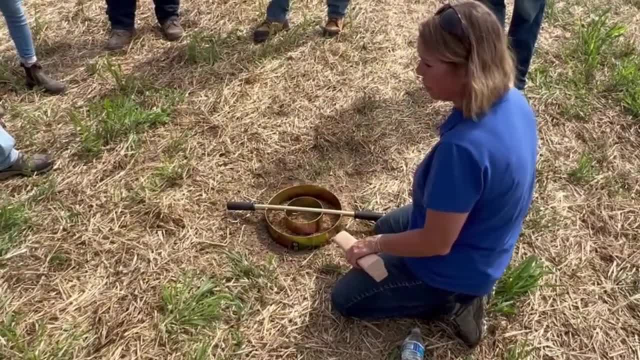 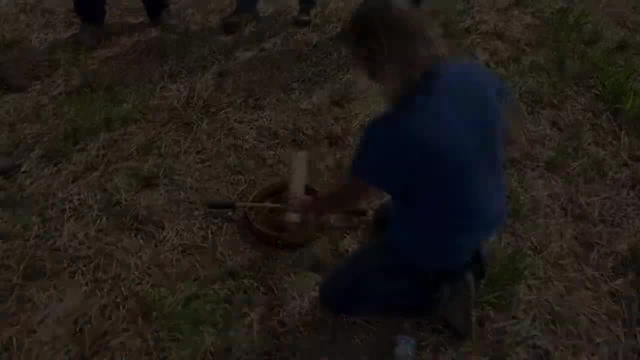 So get a block of wood. Two-by-fours tend to. if you hold it on the side of two-by-fours, it'll hold up a little better. Two-by-fours tend to break apart. So you're going to lay that block in and you're going to pound- well, not on the handle, but you guys won't have a handle. 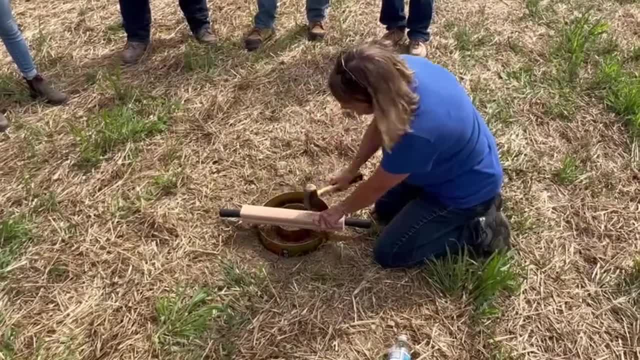 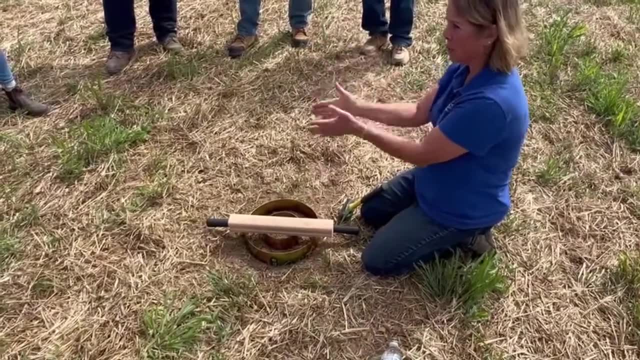 You're going to pound as evenly as you can into that, and I'm just doing that for demonstration purposes. But you don't want to try to rock it. You want to try to get it as straight down as you can and then, after you've got it set, it should be a little bit deeper than this. 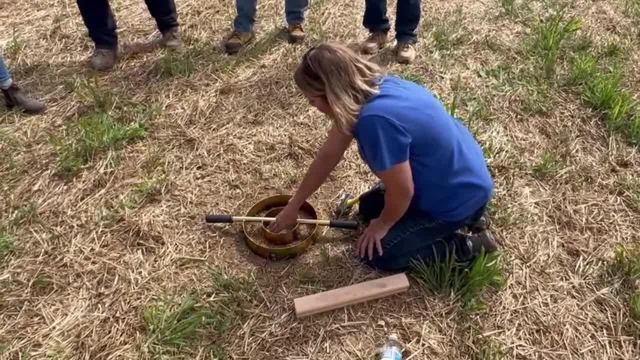 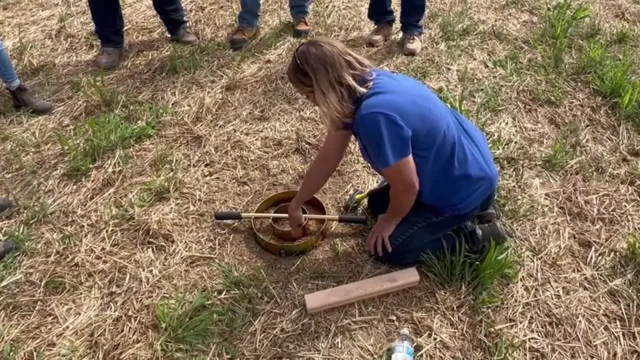 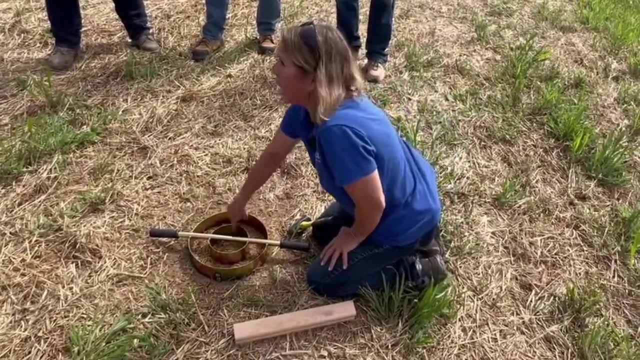 But, like Lee said, the soils are just really dry and challenging. You want to then go around with your fingers and just lightly press the soil against the edge of that pipe, Because what we don't want happening is, when we pour the water on, if we've got gaps right along the pipe. 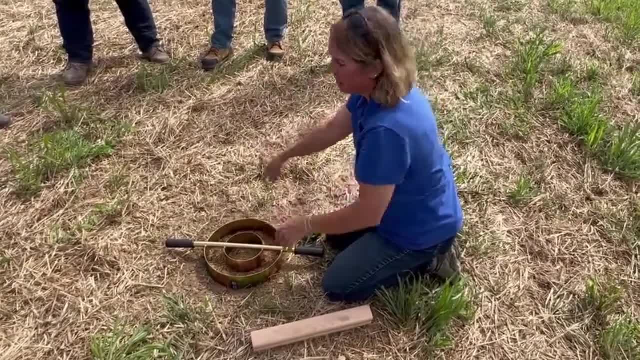 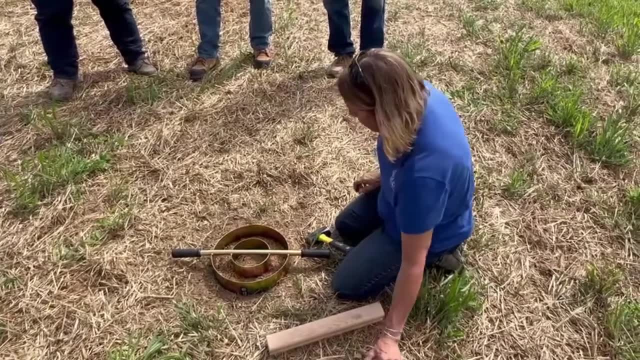 that water's going to just follow that pipe down the sides. So we want to seal those gaps as much as we can so that we're getting a true kind of soil infiltration measure. All right, anything I forgot on that one, You're doing good. It's time for time for rain. 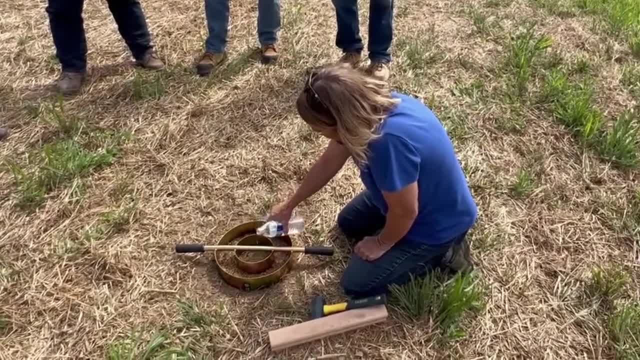 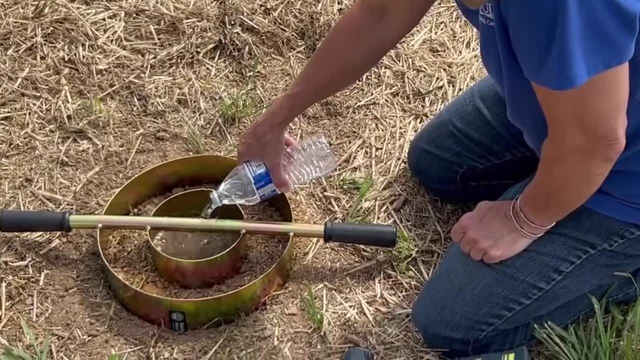 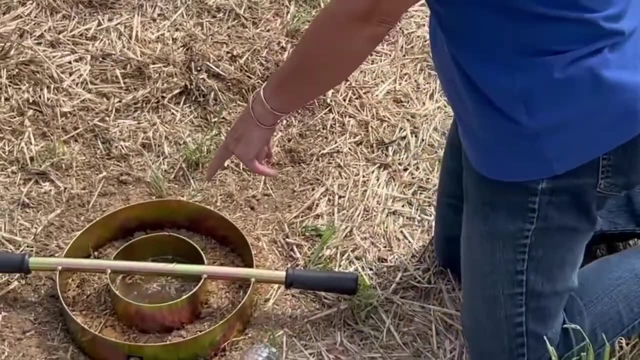 So I'm going to pour this directly on the handle, so we're not kind of pouring it directly on the soil. But oh, we didn't set the time watch, So everybody's normally. I got it. So on your phone you can start the timer. 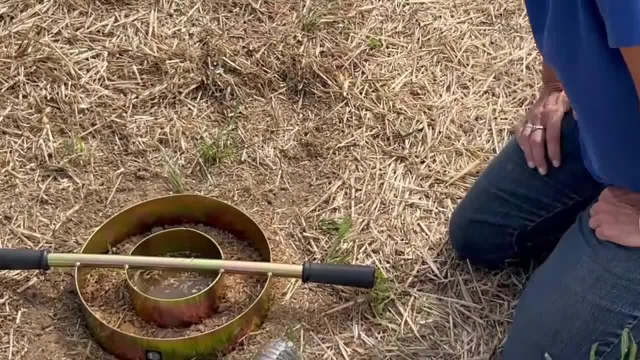 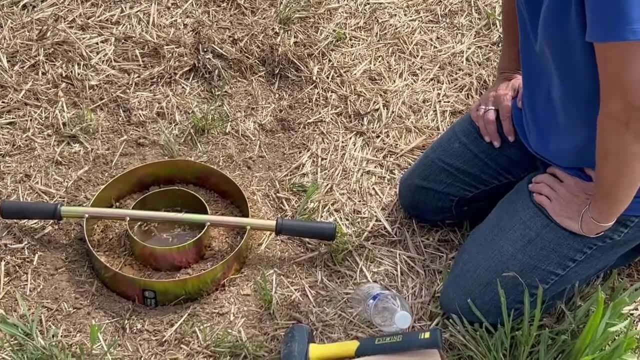 Okay, Okay, When the water gets in there, and then we're going to wait for that water to soak in and we're going to time it on our phone And, this being a real dry soil, right, we're kind of pre-wetting it at this point. 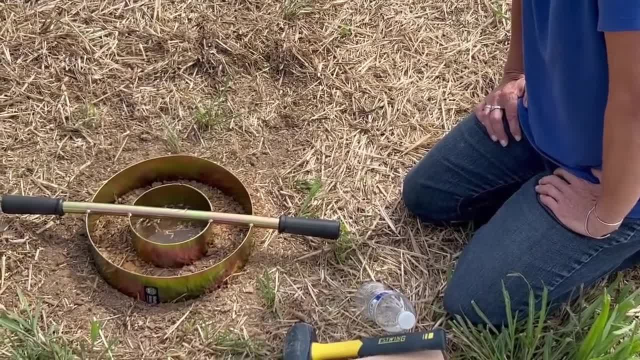 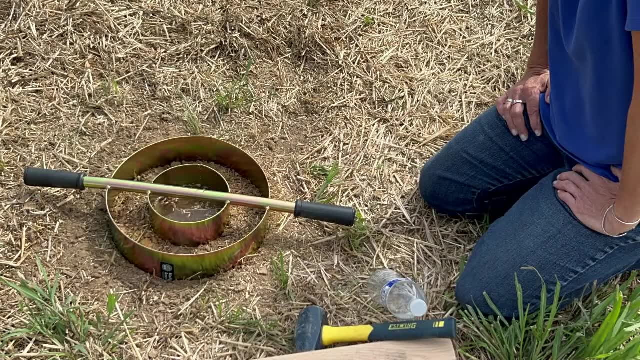 So I bet we'll put a second inch of water on. I bet after we kind of pre-wet with this first inch, we'll see some better infiltration rates. After you've pre-wetted the soil and allowed it to infiltrate, wet the soil again with an inch of water, as Lisa described.